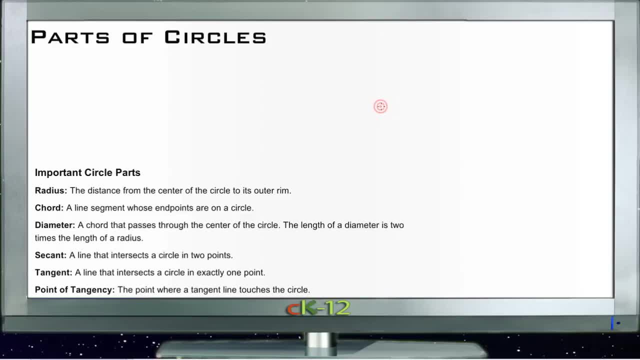 that's not what I wanted. Let's try that again. Let's try U. Is that going to work? Ah, there we go. Good, So here's a circle and we want to start with the radius. So the radius starts at the center of a circle and it's a straight line that runs from the center to any point. 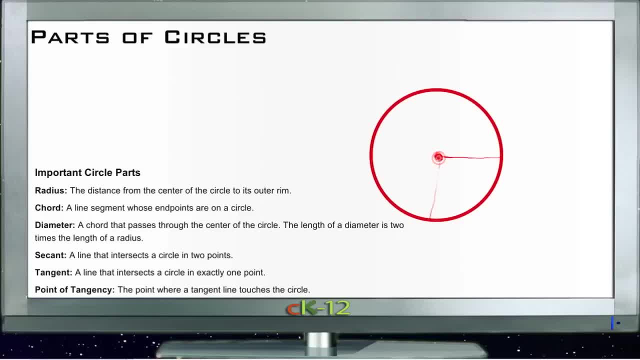 on the circle And, of course, the radius is the same everywhere, because that's the definition of a circle. A circle is, by definition, all of the points that are the same distance from any given point, and we call that given point the center. So radius, which is usually specified by an 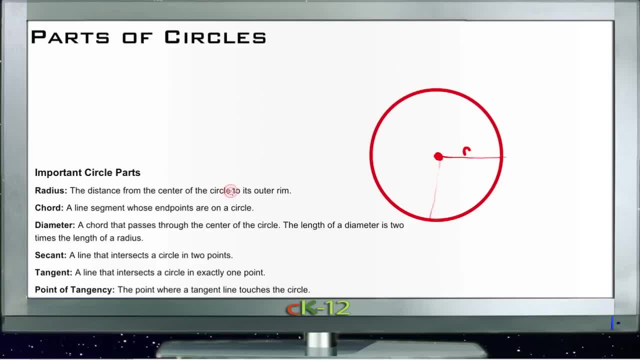 R is that distance from the center out. Now, a chord is a line segment that runs between any two points on the circle. So a chord looks like this. Let me get my straight line tool. I had it replaced with my circle. There we go. So here's a chord. Yep And H O R D, There we go. The diameter would be. 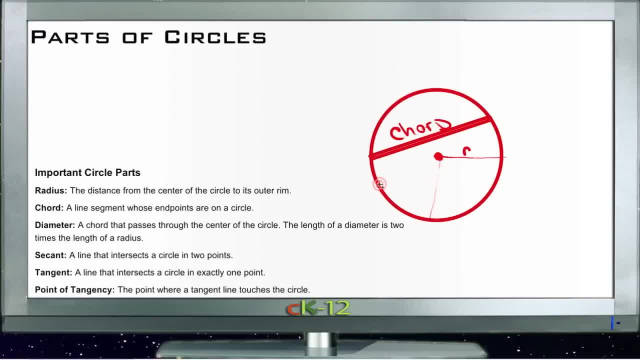 a chord that passes through the center of the circle. So if we have a chord that actually goes right across through the middle, from any point to any point, as long as it goes through the middle, that represents the diameter, And the diameter is usually abbreviated with. 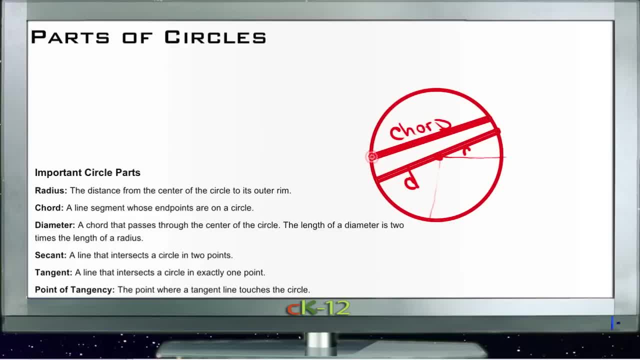 a D Yep. So a secant is very similar to a chord. A secant and a chord are almost the same thing. The only difference is that a secant line doesn't actually stop at the edges of the circle. It's an actual line that goes clear through the circle and out the other side. 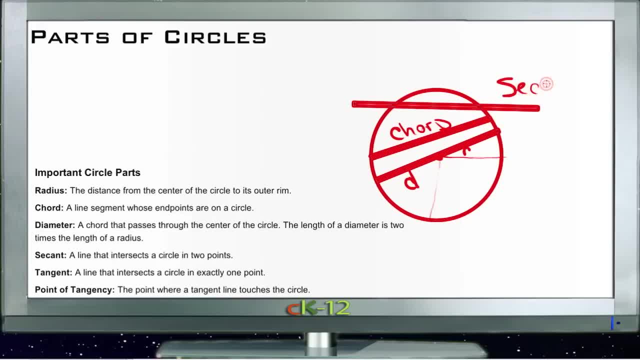 So here's an example of a secant line right here, And you won't see a whole lot of those until you get more into trigonometry. but it's good to know the term and what the difference between a secant and a chord is. If you just draw arrows on the end of a chord and show 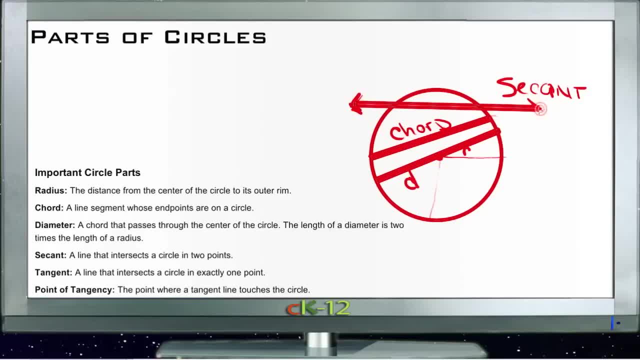 that it goes on forever. then you've sort of turned that chord into a secant line, A tangent again tangent very similar to a chord or a secant. The only difference is that a tangent just touches the circle in one place. So if you have a line that comes,